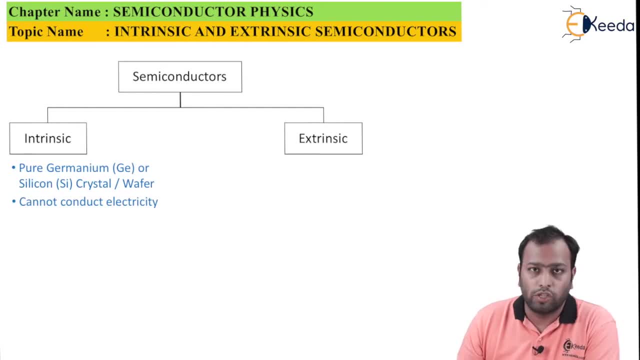 Where it cannot conduct electricity. Now, this could be an important question for your wafer: Why intrinsic semiconductors are incapable of conducting electricity? Well, this is mainly because they do not have any free carriers. Well, you've been learning this in previous classes as well. 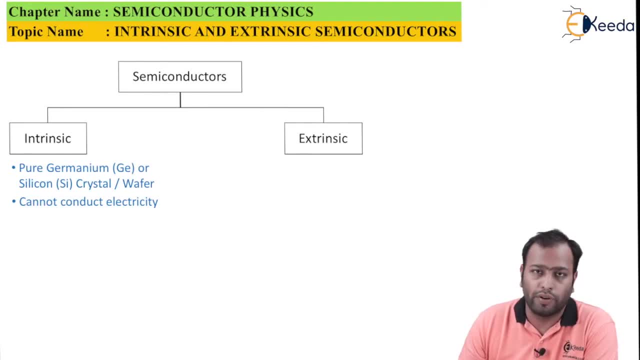 For conduction of electricity, you either need electrons or free ions. Well, in an intrinsic semiconductor, there are silicon atoms and germanium atoms bonded with covalent, So there is no space left for free electrons. So hence you can conduct electricity. 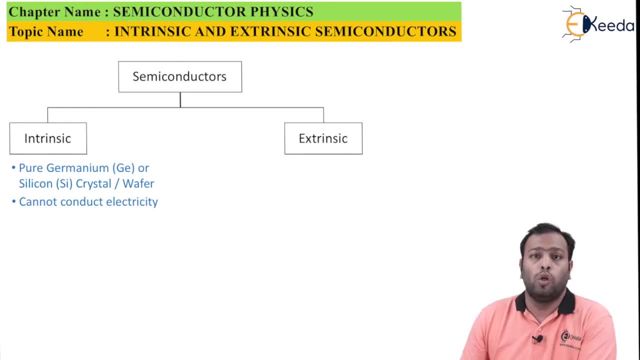 So you can conduct electricity. So you can conduct electricity. Now, what if intrinsic semiconductors are not capable of conducting electricity? Well, if intrinsic semiconductors are not capable of conducting electricity, then how do we use them? 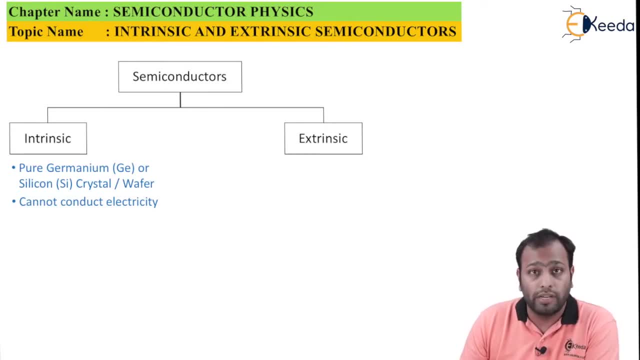 Well, we dope them. Now, if we add impurities to the semiconductor, it becomes an extrinsic semiconductor. So an extrinsic semiconductor is nothing but as a pure germanium or silicon which is doped. Now, what do you mean by doped? 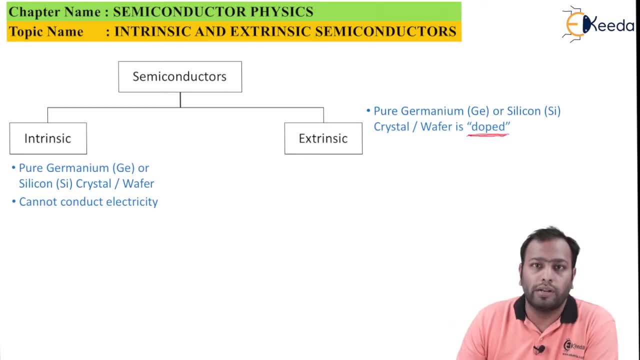 Doped means adding impurities. Now these impurities are just just the same. as we studied in the crystallography chapter, We added some extra foreign materials into the crystal. Well, if you have been adding an extra foreign material, 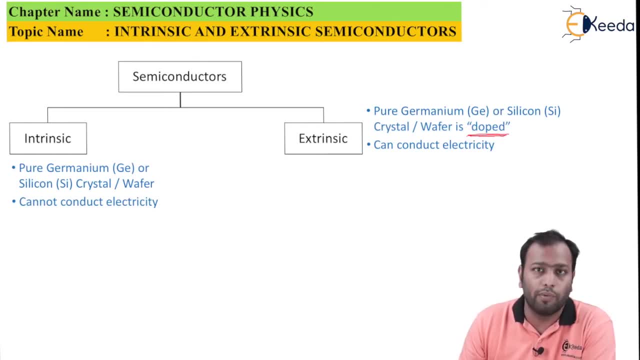 your intrinsic semiconductors becomes extrinsic semiconductors, and now it is capable of conducting electricity. Well, there's an important point to note here that, depending on the amount of impurity that you have been adding to the intrinsic semiconductor to make it extrinsic, 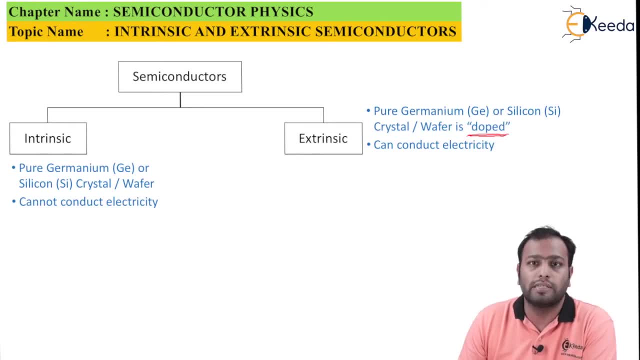 your conductivity depends. Let's say, suppose, for an example, if you have an intrinsic semiconductor and you are adding 10 impurities, so the conductivity would be proportional to 10.. If you are adding 100 impurities, your conductivity will be more than what you have been doing with 10.. 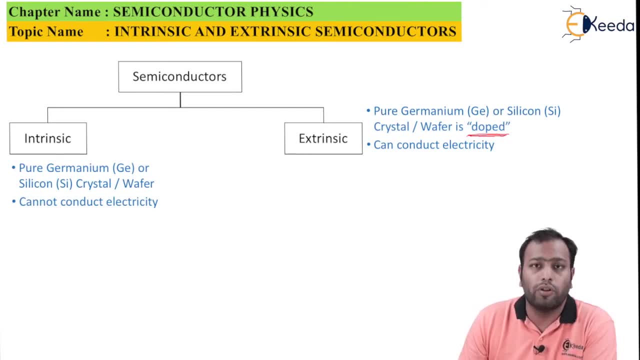 So hence you should make a note that the amount of impurity is directly proportional to the conductivity. Now, extrinsic semiconductors are further classified as two types. You have n-type and p-type. Now, what does this n-type and p-type stand for? 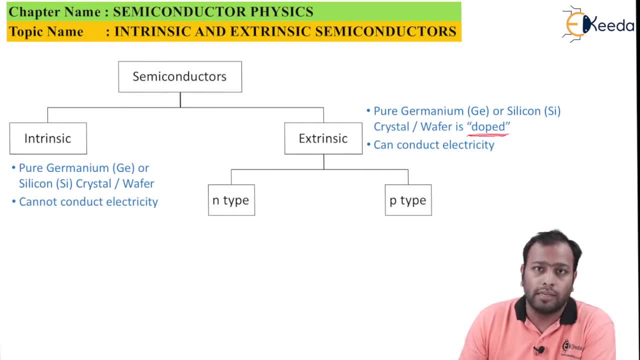 Well, this stands for the majority carrier it has. So what is an n-type semiconductor? Well, it's a pentavalent impurity added semiconductor. Now, what is pentavalent impurity? Well, pentavalent means 5,. 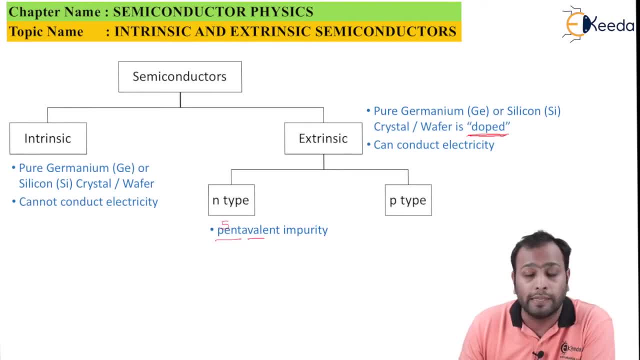 pent means 5, and valent means valency. So basically, in silicon wafer or germanium wafer, I'm introducing an element with 5 electrons. Now what will happen if I add with 5 electrons? Well, we'll be seeing this in the next coming slide. 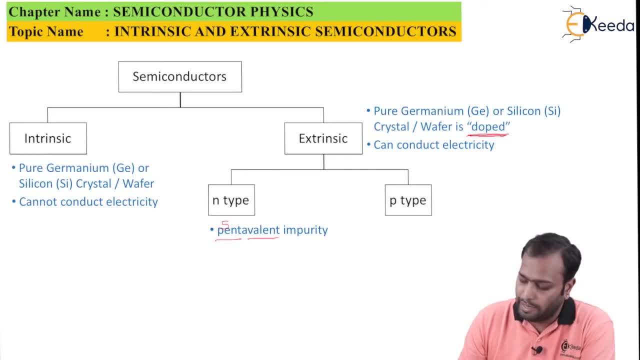 So if n-type is pentavalent, what is p-type? Well, of course it has to be trivalent. tri means 3 and valent means valency again. So key point to remember this is: in n-type semiconductor you add a pentavalent impurity. 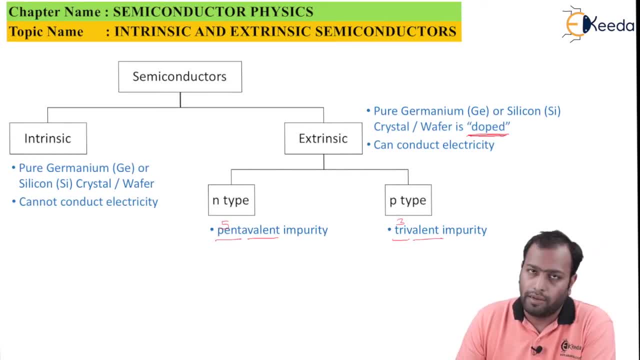 whereas in p-type semiconductor you add a pentavalent impurity, you add a trivalent impurity. Now, what are the elements that are categorized to have pentavalent impurities? Well, these are the elements as nitrogen, phosphorus, arsenic. 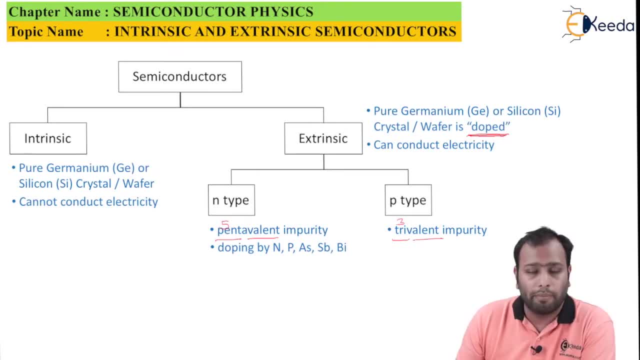 Sb and bismuth. Now for what about trivalent impurities? Well, the elements here are boron, aluminium, gallium, iridium and thallium. Now, these are the impurities that you add to make. 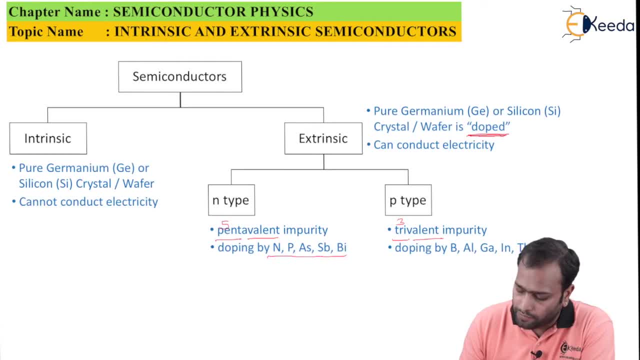 p-type, and these are the impurities you make for n-type. Well, these are the impurities you make for p-type. Now, the majority carriers here in n-type are electrons, and holes are the majority carriers for p-type. So, in a nutshell, now you know about n-type, semiconductors are the 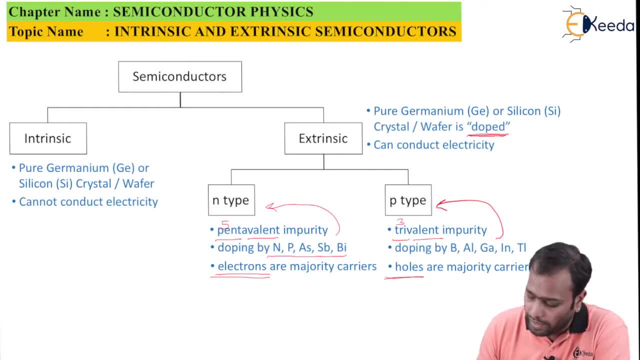 semiconductors which are doped with pentavalent impurities. The materials include n, p As Sb and Bi, Whereas electrons are their majority carriers. However, in p-type semiconductors it's trivalent impurity. 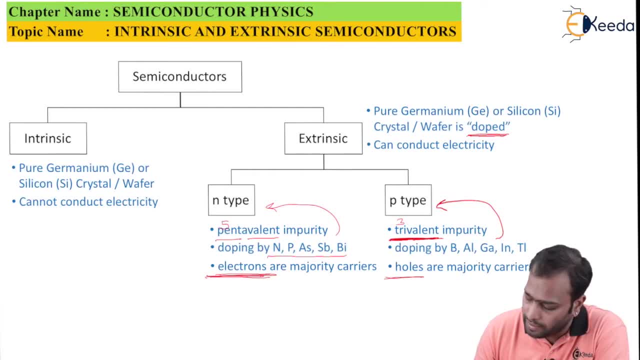 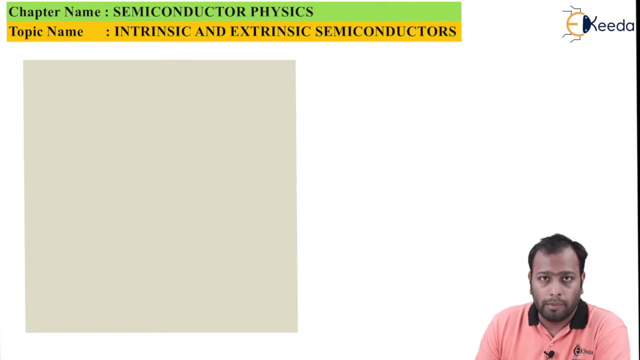 that makes the p-type semiconductor, which includes B, Al, Ga In and Tl, and holes are the majority carriers. Now let's see in detail what an intrinsic and extrinsic semiconductor looks like. Now you have a plain wafer of silicon. How does the silicon looks like? Well, this is the silicon. 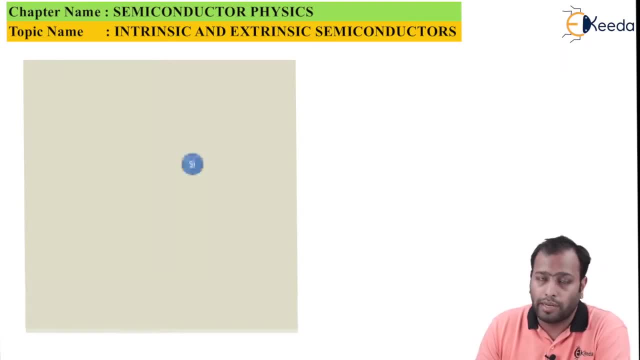 and I'll be drawing the outer electronic configuration, as you all know that it has four electrons in the outermost shell. So this is the outermost shell and it has four electrons: one, two, three and four. Now, there won't be, of course, only one single atom of silicon in the 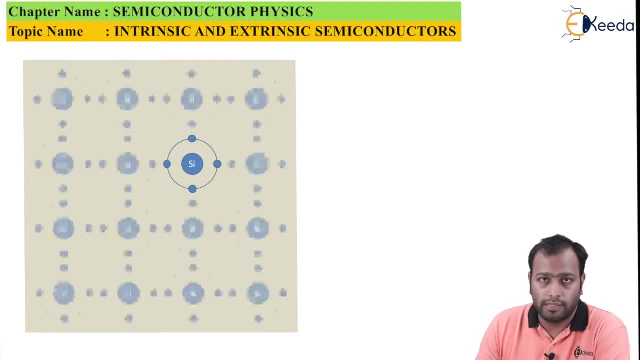 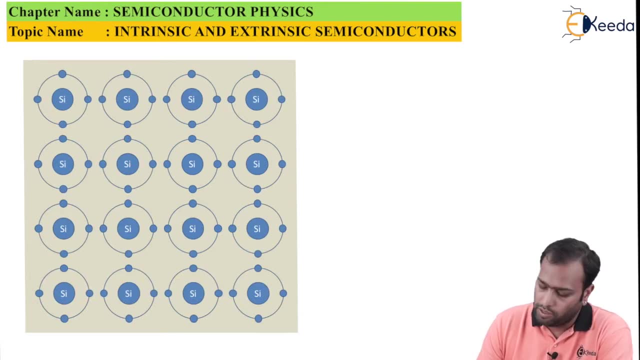 wafer. There would be many others, So here it is. Now every silicon atom will be forming a covalent bond with the neighboring silicon atom, So here is the bond that has been formed. As you can see, this silicon atom is forming four covalent bonds. Now this would replicate across the entire. 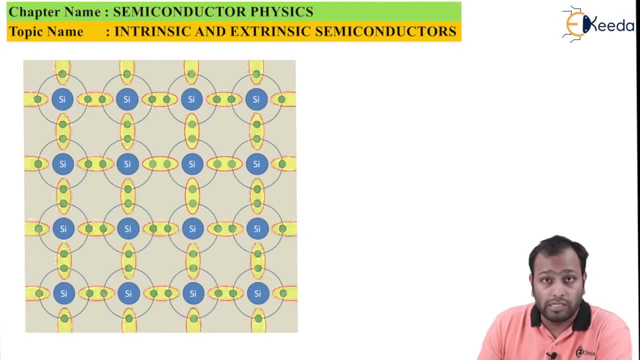 wafer, and this is how it's going to appear like. So this type of semiconductor, as you can see, there are only silicon atoms and hence it is called as an intrinsic semiconductor. Intrinsic means pure, It means it has no impurities or no doping. Right Now let's move ahead. 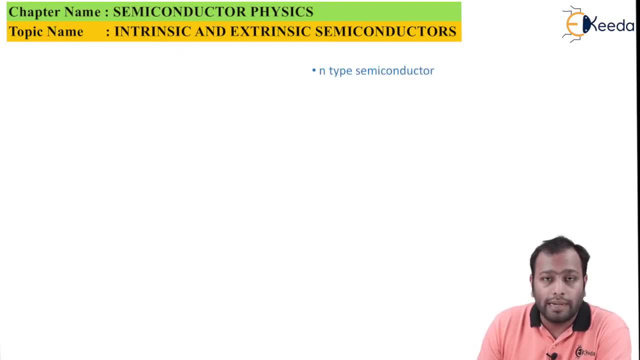 How I'll make a silicon semiconductor. Well, I'll make a silicon semiconductor. How I'll make a silicon semiconductor: Well, I'll make a silicon semiconductor. How I'll make a silicon semiconductor: Well, as you know, n-type semiconductors are made by using. 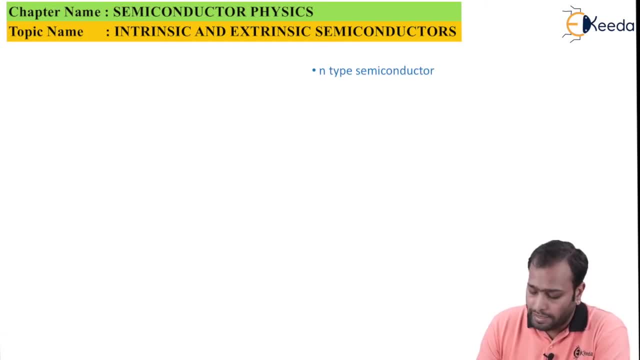 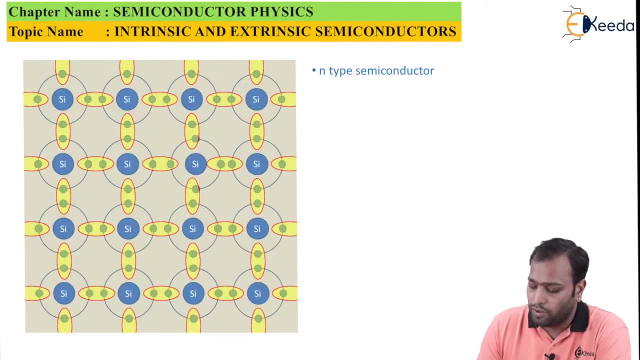 pentavalent impurities. So I'll be taking this, which is nothing but as an intrinsic semiconductor or the pure semiconductor, I'll remove the silicon atom from the wafer and I'll introduce phosphorus. Now, what is phosphorus? As you know, the outer electronic configuration of 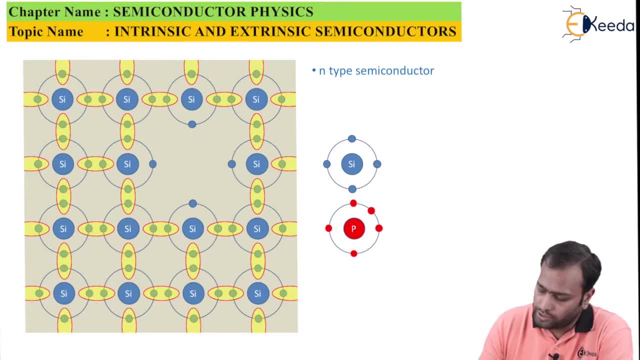 phosphorus says that it has five electrons in the outermost shell. I'll replace this removed silicon atom with phosphorus. Now, as you can see, the site of silicon which was removed is being now taken by phosphorus. It can form four covalent bonds. 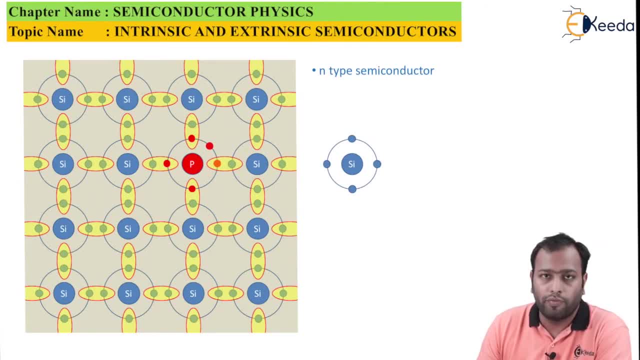 of course, with the silicon, the neighbourings, It is now left with one electron which is not there for bonding. Now this electron will continue to move throughout the wafer. Well, if you add more phosphorus atoms, there would be more number of free electrons that would be available for. 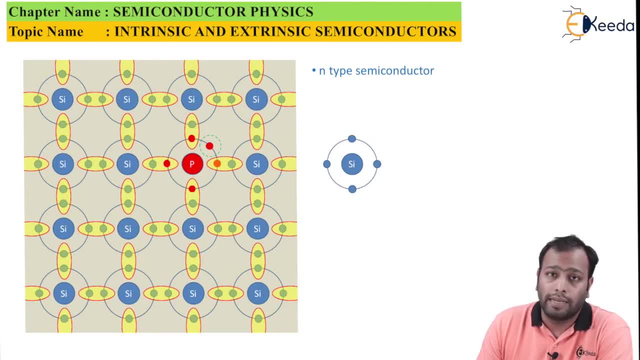 conduction. Well, this statement proves that. yes, it is true. The more amount of impurity you add to an intrinsic semiconductor, the more conductivity you get. So basically, this could be an important question for Aviva. Conductivity of a semiconductor is directly proportional to the impurity added.